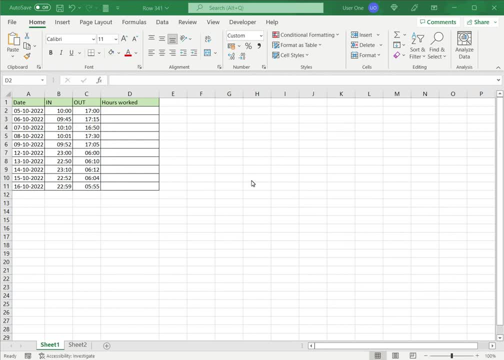 How to calculate hours worked in Excel using a 24-hour clock. Excel treats date and time formats differently from numbers and text because of the different scale that dates and times used. We have 24 hours in a day, 60 minutes in an hour, etc. So when I format a date and time as a date and time, I can 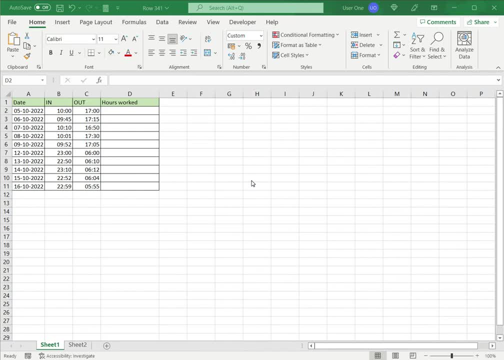 perform basic mathematical operations such as addition and subtraction. So here we're going to see how to calculate the hours worked. I have a timesheet of an employee Now. in this one we see that for the first week the employees worked a day shift, but from the second week onwards the employer shifted to the 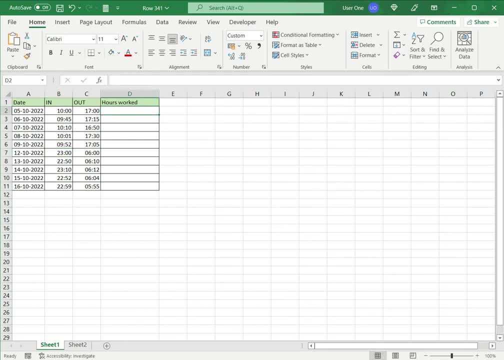 night shift. Both these times are formatted as times, so I can just apply basic subtraction here to get the hours worked. I subtract the out time from the in time and I get seven hours. So this works fine, as long as it is during the day and the end time. 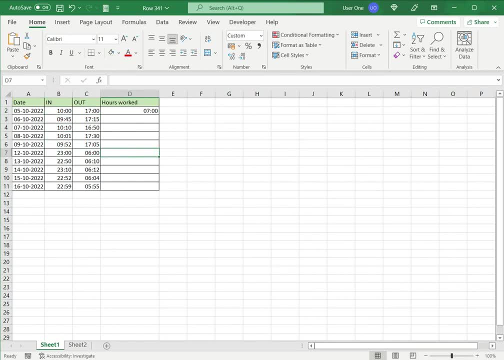 The out time is greater than the in time, but see what happens when I cross over into the next day. So the out time becomes lesser than the in time. Okay, so now Excel is not able to handle this, So there is a workaround for this. 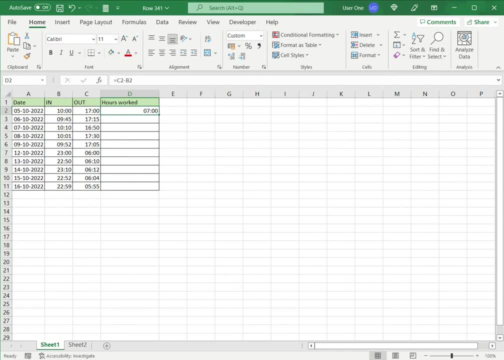 to indicate that you know to get the correct value, and this is by using the mod function. The mod function returns the remainder of the modulus of a number that is divided by a divisor. So let's do that here. I will say: let's delete this and type the mod function and 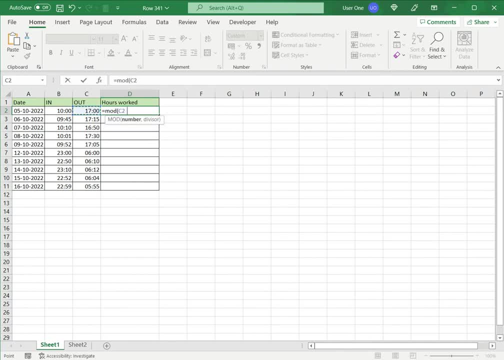 now the number I want is this formula, and I'm going to just divide it by 1.. So we know that when you divide the number by 1, it will remove the negative part of the number and I'll say: enter. Now. of course, this has no change for the 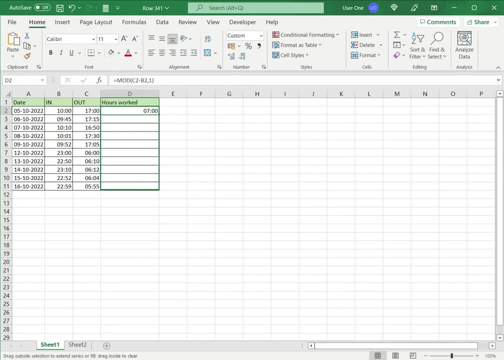 first record, since there was no issue there. but when I drag this down I can see that it works perfectly even for the night shift timings, because it is able to just take the difference between these timings and I get the correct values here. So this: